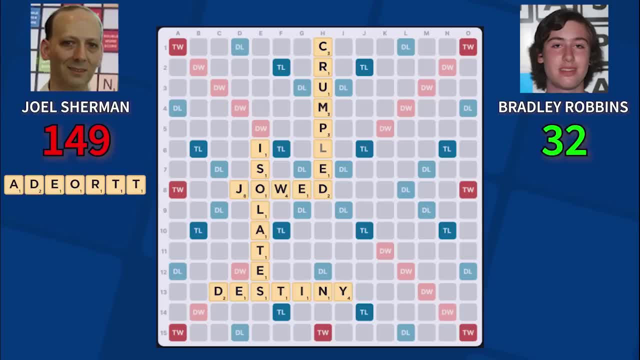 Bradley's solid response of Destiny for 32, Joel bingos a second time with Outrated for 72. He had Outtrade in the same spot for the same score, but he likely picked Outrated to avoid giving Bradley unnecessary hooks. on the triple lane, Bradley draws the X and plays a heavy-hitting Wax. 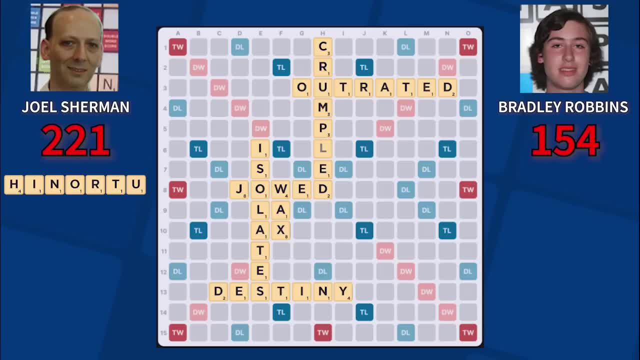 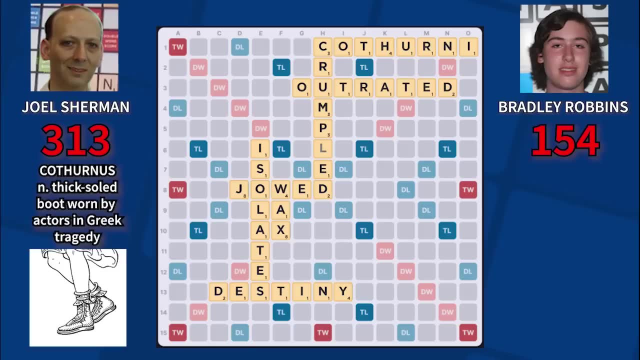 for 56,, but Joel's onslaught continues with the beautiful play of Cotherny- the plural of Cothernus, the thick-soled boot used by actors in Greek tragedy. Bradley plays Pence for 30,, bringing his score to a respectable 184 after five turns, one of which was an exchange. 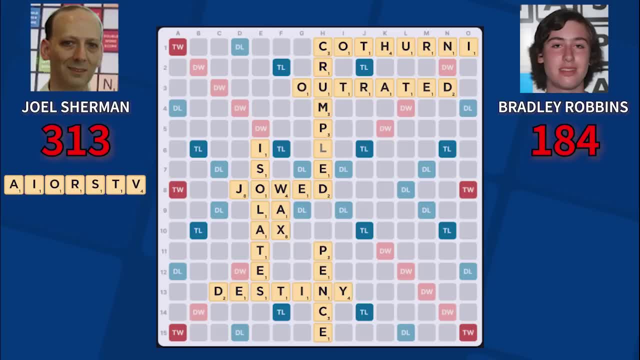 but there's nothing he can do about Joel playing his fourth bingo in a row, with Travoise for 95 points, Giving him over 400 points with roughly half of the game still to play. But this scoring pace is completely unsustainable, right? Well, let's find out. After Bradley's coy for 21,, Joel has an. 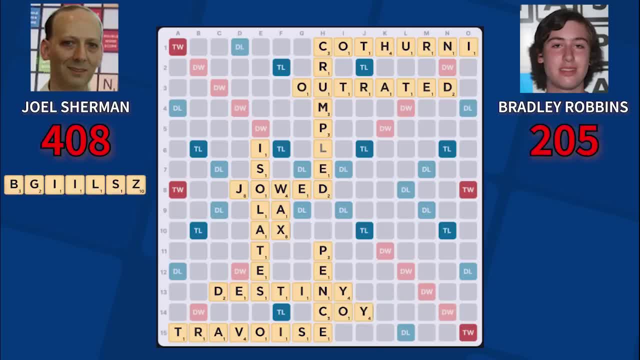 interesting choice Holding the Z. he makes a very clever play here of Glib for 18, setting up a huge spot to cash in his Z next turn with Biz for over 60 points, which is a very good play. Bradley is struggling with vowels and plays Ulu for just three points to balance his rack. It also 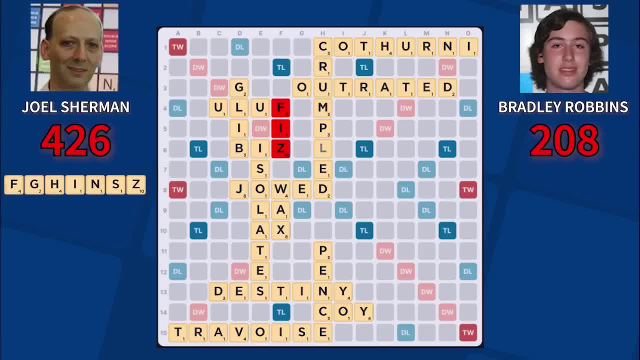 blocks Joel from playing the Z spot, which is a very good play. But this scoring pace is also failed to help Joel from cashing his setup with Fizz and Biz for 69,. but he has a solid option in Fez, keeping the synergistic S-H-I-N-G. Joel draws A-K to that combo to threaten shaking. 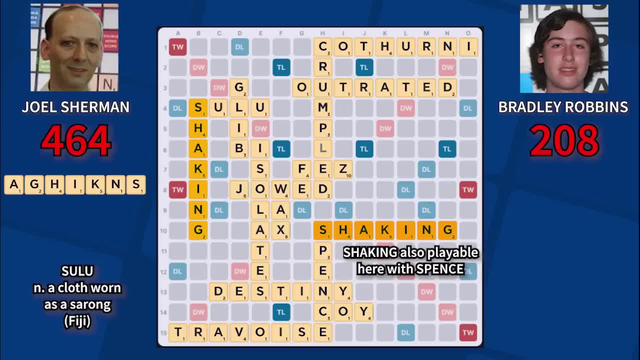 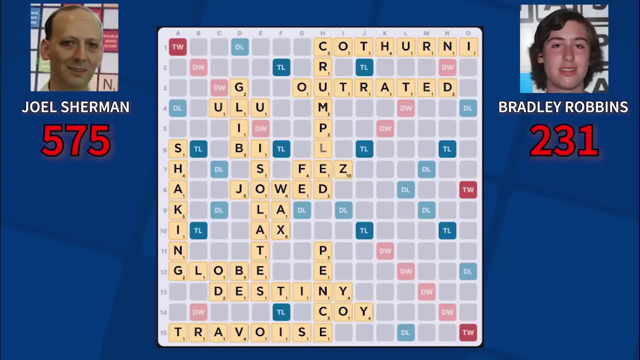 which will play to the S hook, with Ulu forming Sulu. But after Bradley plays Lobe for 23,, which looks entirely reasonable, here Joel has an even heavier hitting spot for shaking hooking globe for a whopping 111 points. Joel's good fortune continues as Bradley exchanges tiles. 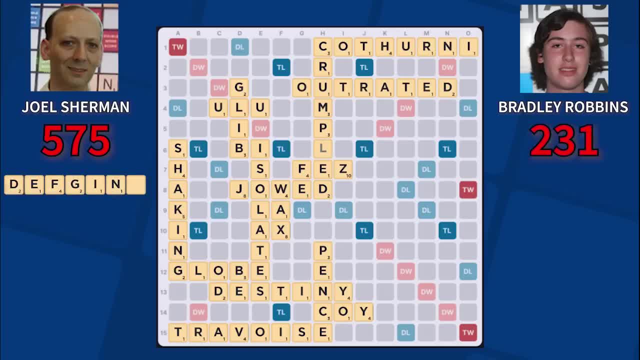 while Joel draws the second blank Without any playable bingos, Joel plays if for 32 instead of diff for slightly more points, acknowledging the vowel overload in the unseen tiles and keeping an extra consonant After Bradley plays. nada to dump two more vowels. Joel plays his only available. 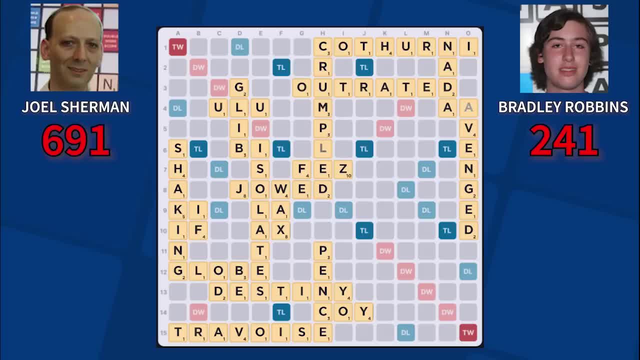 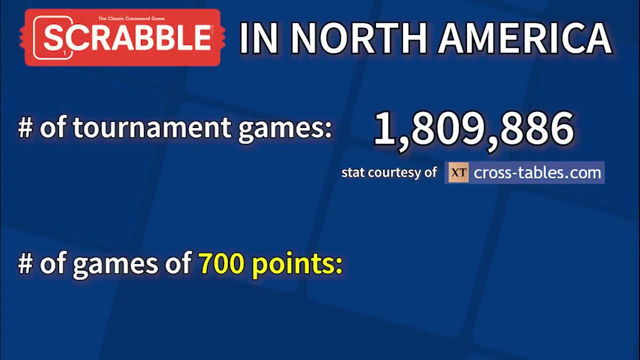 bingo of avenged for 84,, bringing him within striking distance of 700 total points. Keep in mind that in the nearly 1,810,000 games of Tournament Scrabble played in North American history, only 55 of them have featured a player scoring 700 points or more. so this is an 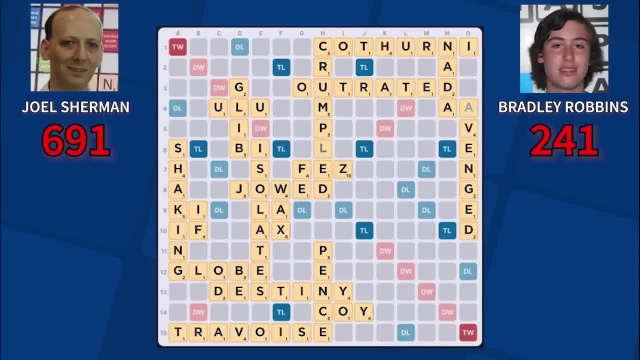 achievement in and of itself. Bradley makes the nice overlap of fem for 30, leaving one tile in the bag and creating a new tile for the other. Bradley is able to block the only spot where the cue is playable. Tournament players call this a. 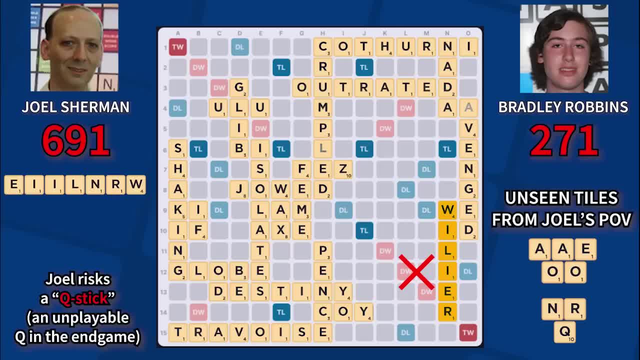 stick and the cue is one of the likeliest tiles to be stuck with at the end of a game. To avoid this, Joel plays- we for 30, and then he plays a little bit of bingos, keeping his eyes to better manage the cue if he should draw it with several spots available to 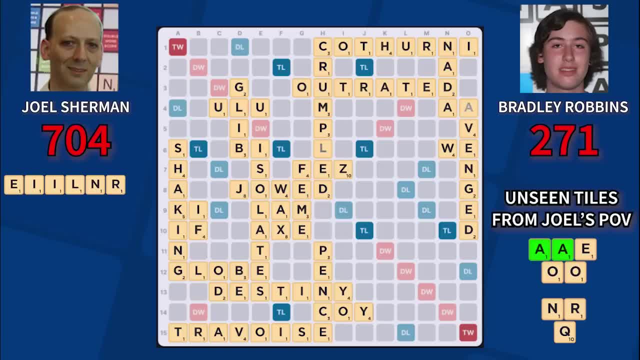 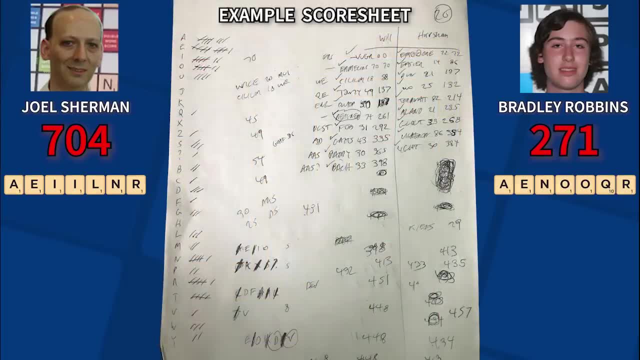 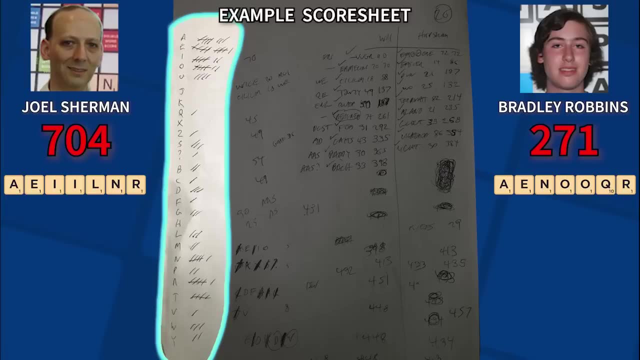 play chi. It also threatens airline with an a draw from the bag, And of course that's exactly what he draws. Normally, players at the expert level carefully track the tiles that have been played so they can strategize more effectively in the endgame. In Bradley's case, he stopped tracking. 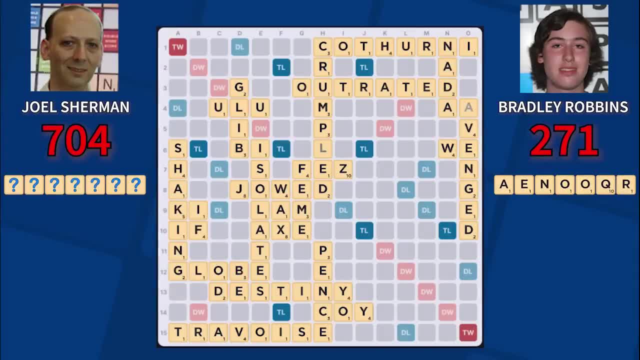 long ago in this game, which I think is a good thing. So if you're a player who's been playing for a long time, you should be able to track the tiles that have been played, which I think is a we should forgive him for, considering Joel was up by literally 400 points. 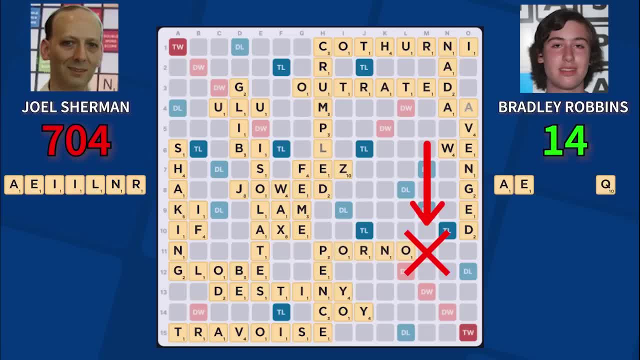 Given this, Bradley plays porno, interfering with the new lane that Joel just opened with we, as well as blocking some possible bingos from the A and T of outrated After porno, one spot for airline is blocked, but Joel is still able to use the other one for a 75 point out bingo bringing. 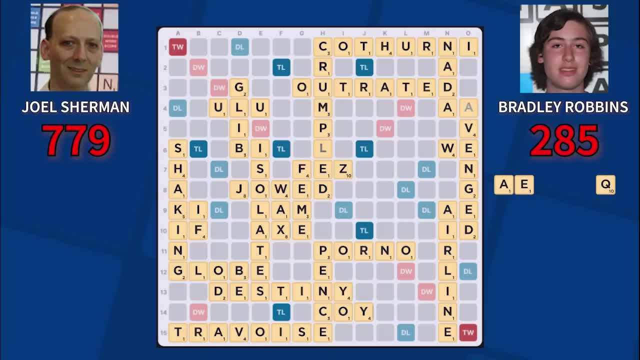 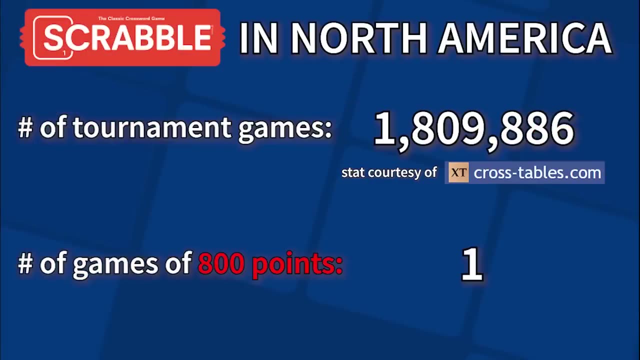 him to 779 points, But he then collects 24 more points from Bradley's unplayed AEQ, giving him a final score of a mind-boggling 803 points. This remains the only 800 point game in North American tournament history. 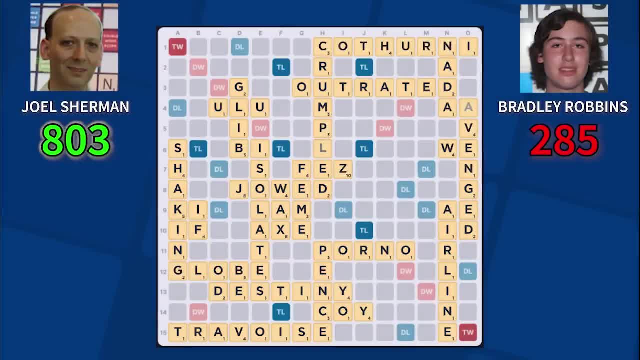 and there's several remarkable things about it. First, all of the words played in the game were valid. Joel didn't benefit from Bradley playing a phony word, incorrectly challenging any of his words or playing a phony word. that was unchallenged. 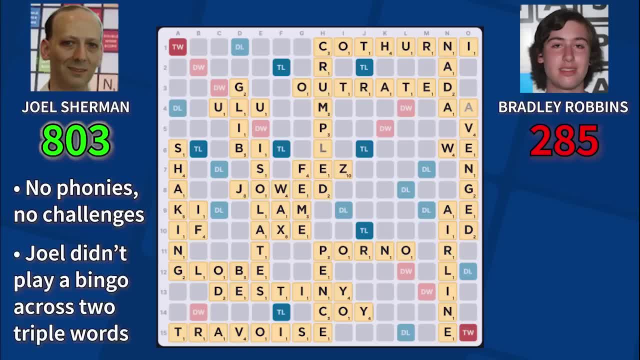 Secondly, Joel didn't play a triple-triple or a play spanning two triple word squares. These are the highest scoring plays in Scrabble and typically to score anywhere near 700 points, let alone 800,, you'd need to land one of these incredibly damaging plays. 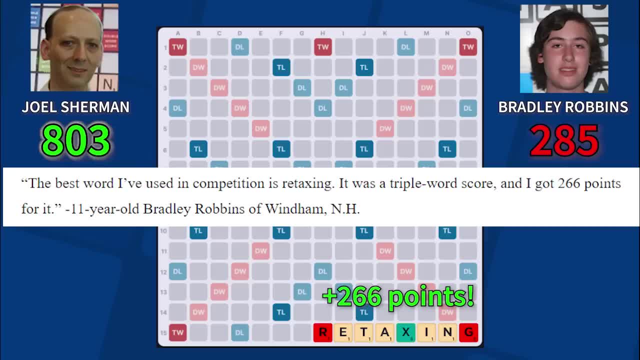 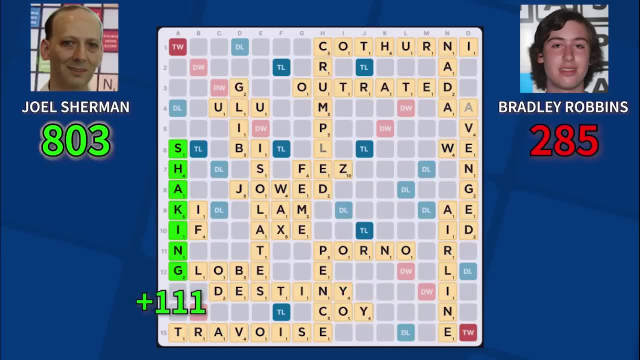 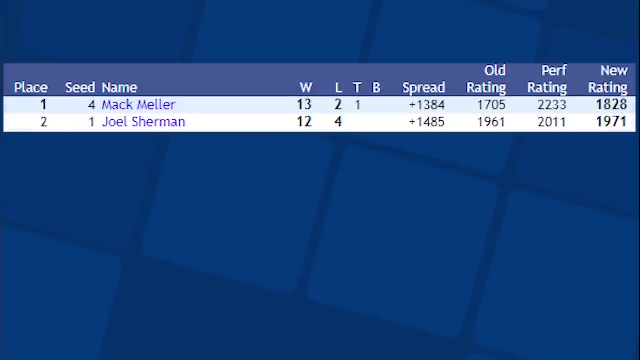 as Bradley himself once did, with re-taxing for 266 points. Joel's highest score in this game was 111 points for shaking, which, while undoubtedly impressive, is shockingly low for a game in which he scored 800 total points. Amazingly, Joel didn't even win this tournament. That honor went to Mac Meller who, at the age of 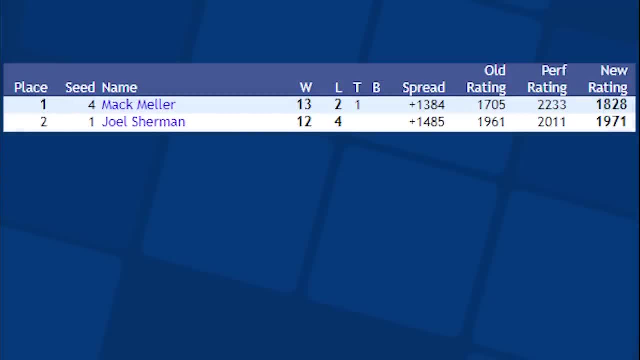 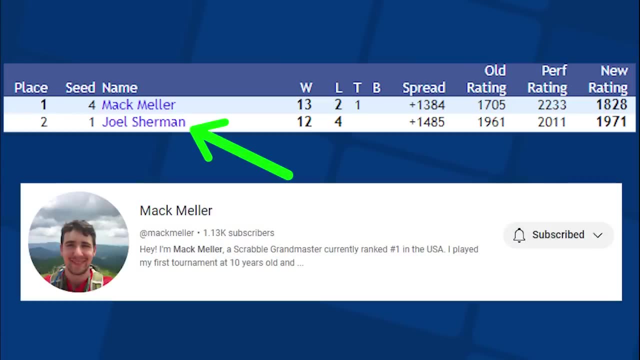 11 years old, became the youngest player in Scrabble history to achieve an 1800 rating. You should go follow him on YouTube. by the way, Joel ended up finishing a close second. But Joel has been long overdue to appear on Scrabble history. 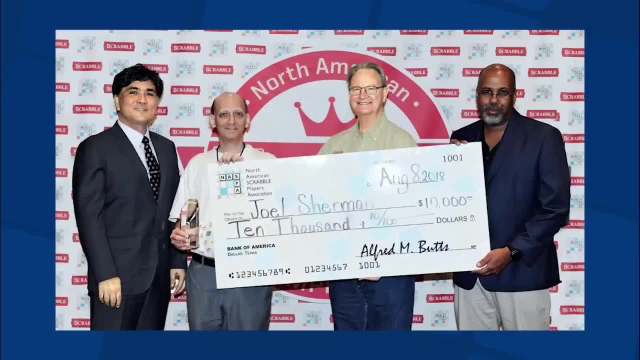 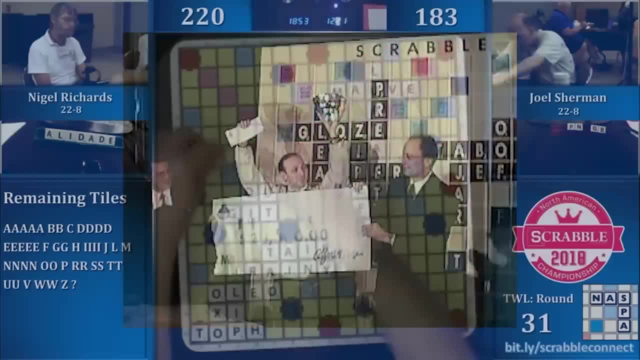 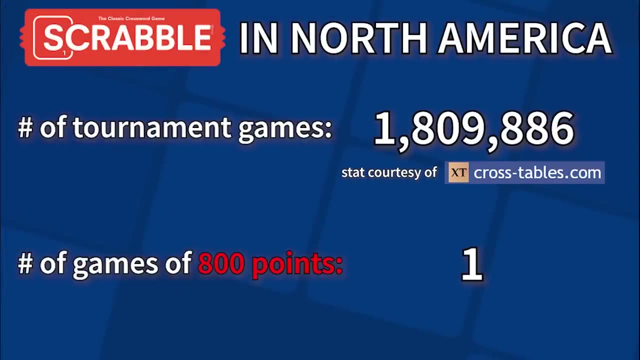 He's etched into Scrabble's record book as the only player from North America to win multiple North American championships and a world championship, and some of his performances in these events are incredible stories in their own right. But it's somehow fitting that Joel Sherman is also in the record book for one of Scrabble's